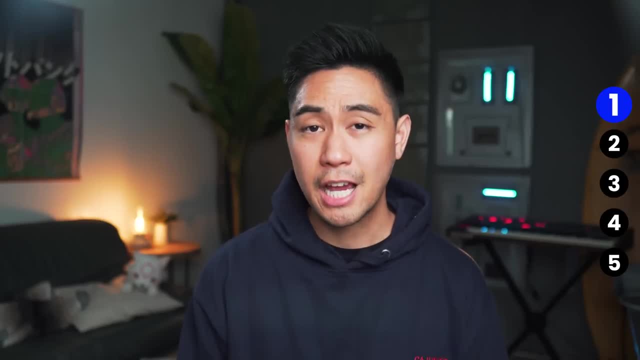 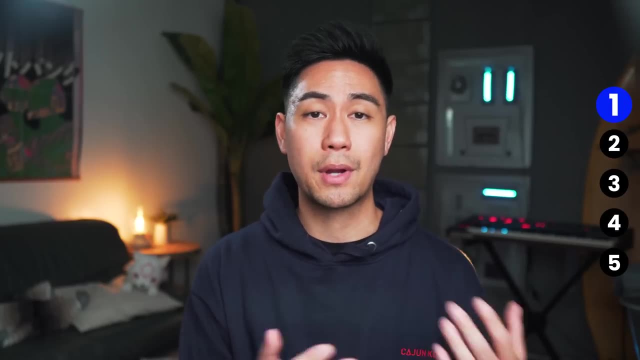 reading assignments or to do 20 flashcards. But after timing myself, I realized that I can get a lot of work done in all the random bits of time throughout the day, like in between classes or on the bus ride home, that would have otherwise been wasted. Next, you'll only need two items to carry. 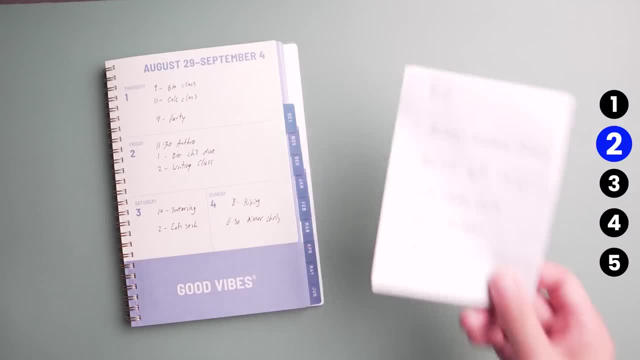 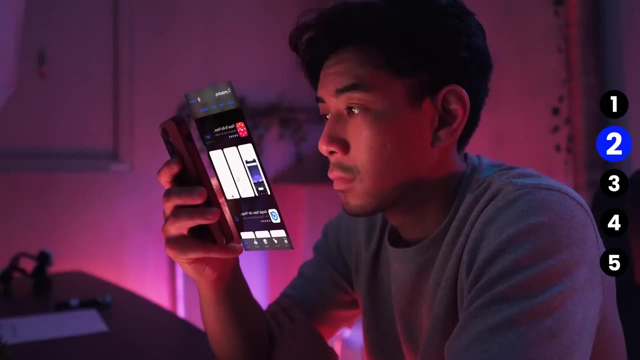 out this entire time management system, a calendar and a piece of paper. Or you can use your smartphone if you have one, But don't worry about all these fancy to-do list apps and routine trackers and stuff like that. If you can master this analog method, then you can later customize. 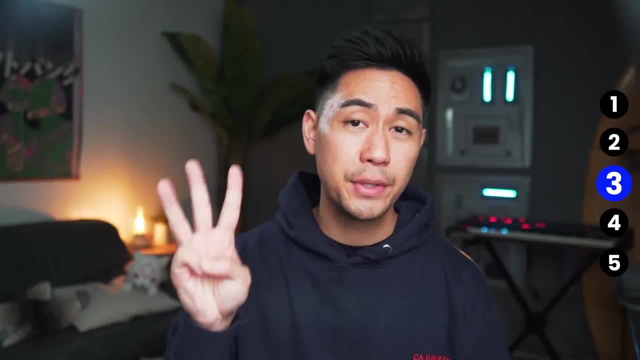 it and make it as sophisticated as you need it to be. Now, there are three steps to this time management system. This is basically the first step. The first step is to make sure that you're doing it right. This is based off of Cal Newport's book, so shout out to him. The three steps are: 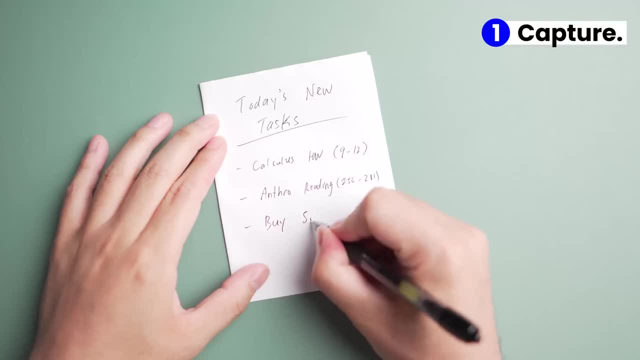 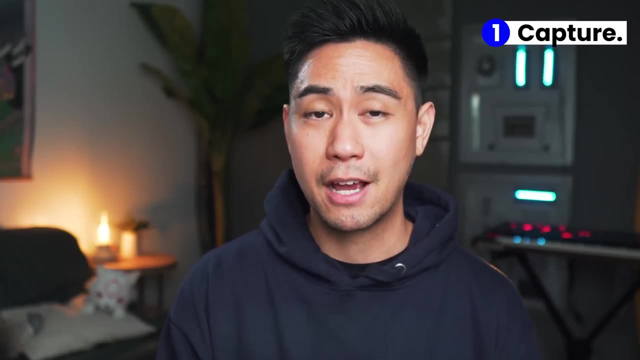 number one. whenever a new task or assignment comes up throughout the day, you want to quickly jot it down on your piece of paper. For me, the hardest part about this entire system is just remembering to write things down on the spot, But the more you do it, the easier it gets. 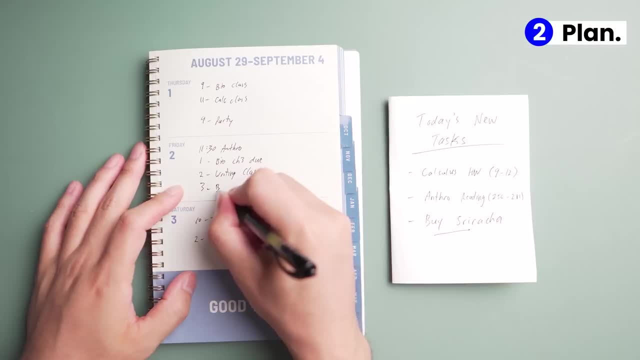 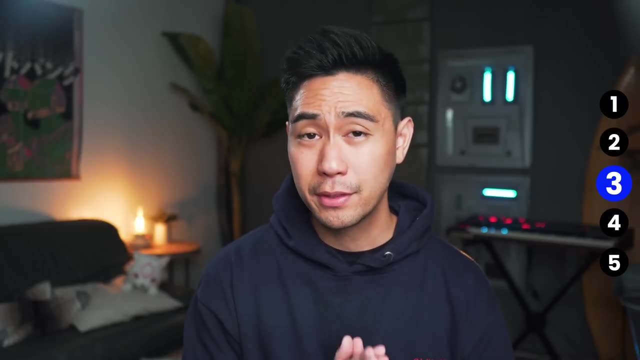 Step two happens the next morning. You want to plan your day based on what needs to be done. And step three is to move all other tasks to future dates in the calendar. So I'm going to show you an example of what the three steps look like in action. 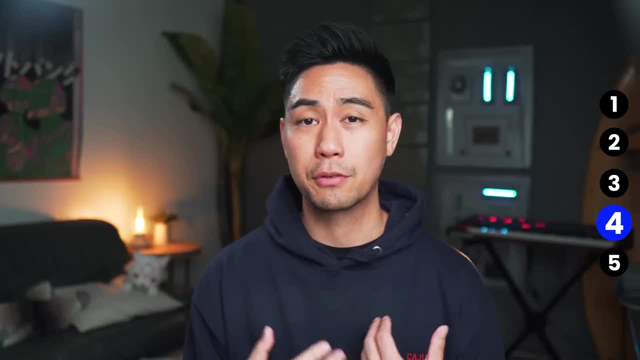 but I want to emphasize four rules that really made this system work for me, especially when I was studying for my dual degrees. The first rule is it has to be flexible. We're not trying to be Elon Musk and plan every minute of our day in order to run four companies. 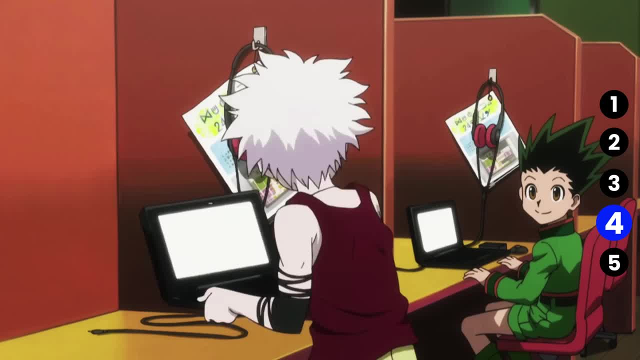 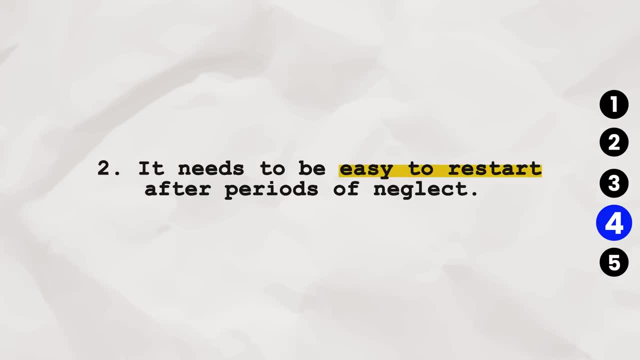 at the same time. We're students. We need to be ready on a moment's notice when our friends hit us up for an impromptu ramen run. The second rule is it needs to be easy to restart after periods of neglect. I love this idea. It's also from Cal Newport. We're human. We're not perfect. 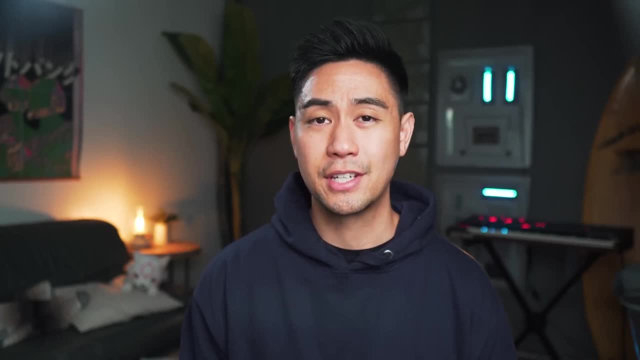 We're going to miss days, and that's okay, But once you've seen how organization can change your life, you're going to have a hard time going long periods of time without it. Number three is it has to reduce stress, And we do this by offloading all the things we need to. 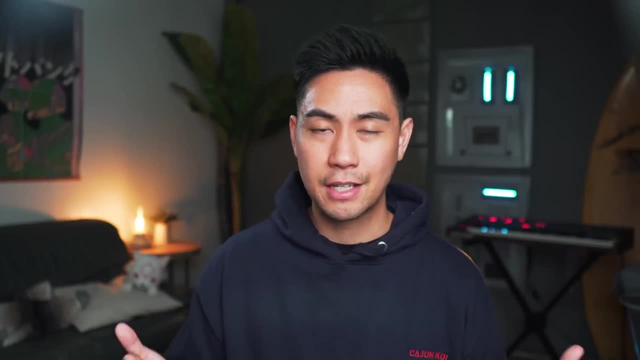 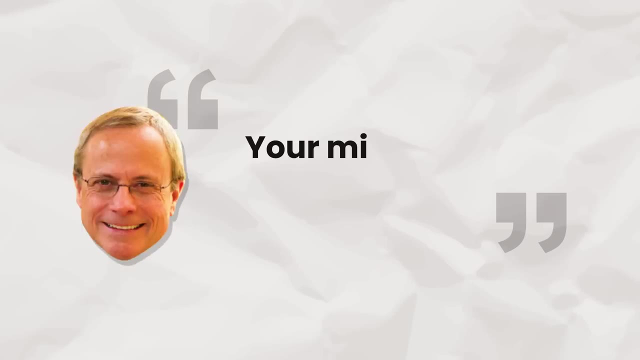 remember onto our paper. Having obligations and deadlines kind of floating around your head is exhausting. Plus, it makes it impossible to relax when you want to. As author David Allen says, your mind is for having ideas, not holding them. So this is why we want to immediately record any tasks or deadlines that we 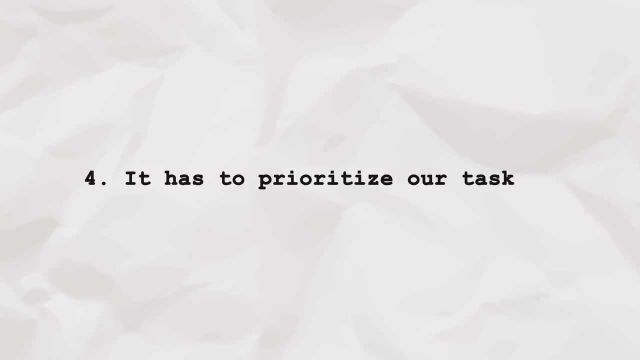 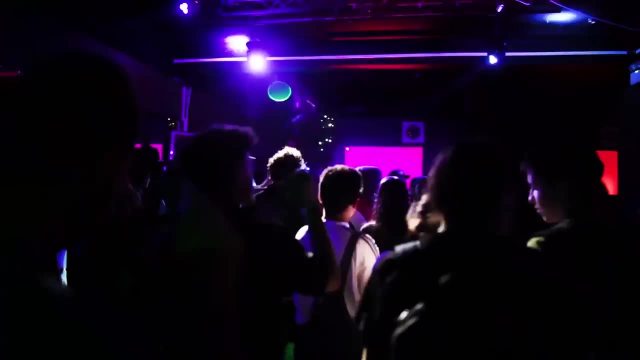 forget and offload them from our brain. And four, it has to prioritize our tasks. It's impossible to do everything. We can't manage to go to every party or join every club. Sometimes it's not even possible to do every single assignment for every class, So we have to. 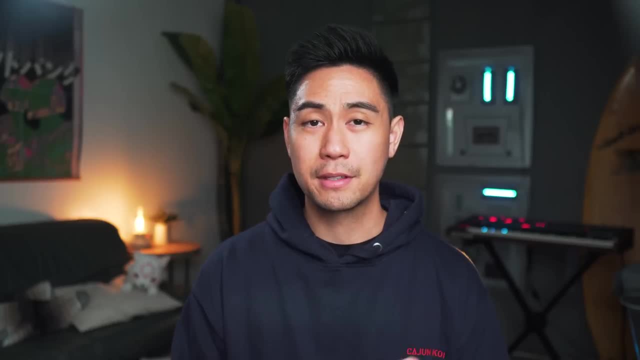 pick and choose what's important to us. So that's why this method consolidates all our options and clearly displays in front of us, so that we can make informed decisions when it matters. With these rules in mind, let's look at a typical Thursday for young college Maddie. 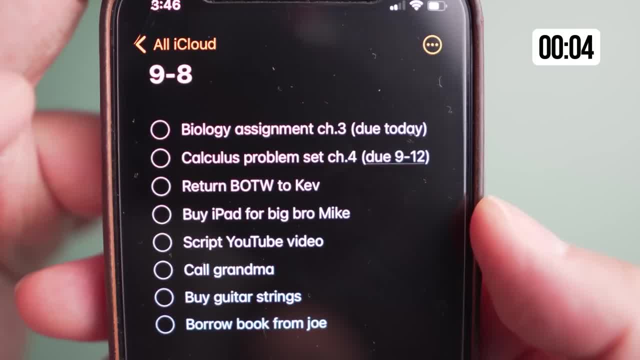 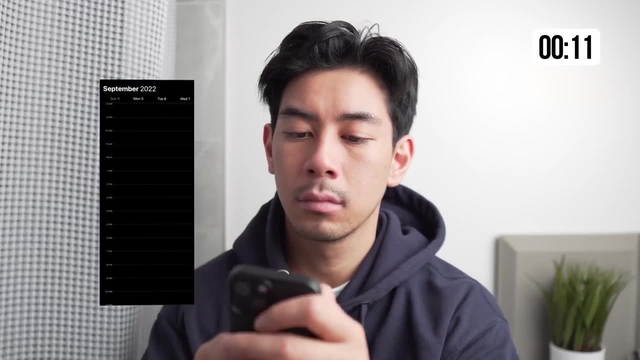 Maddie wakes up at 8: 30 am for class at 9.. He starts by pulling out his list from yesterday containing all the tasks that he had recorded throughout the day. Now he looks at his calendar to see what's already been scheduled. He has class at 9 and 11 am. There are dinner plans. 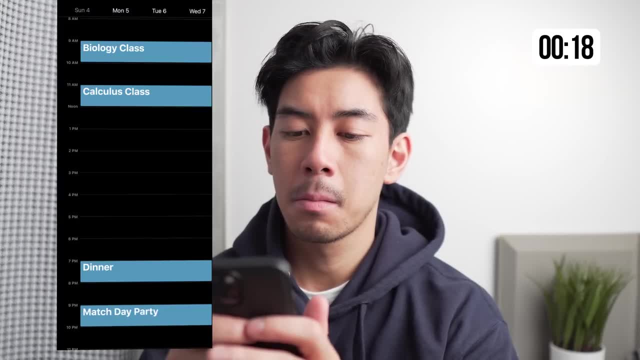 with his friends at 7 pm, Then a party for the newly matched rookies at 9 pm. He wants to go to the gym before dinner, so he plans to have all of his schoolwork done by 5 pm. Now he. 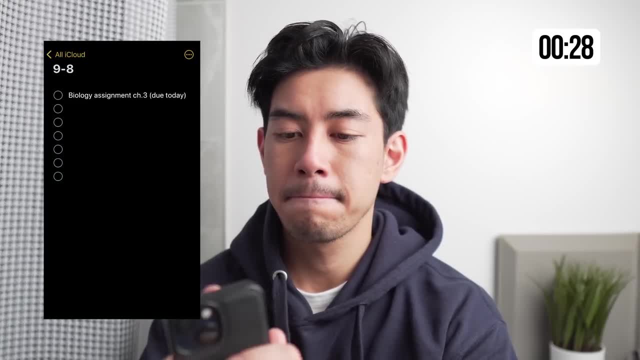 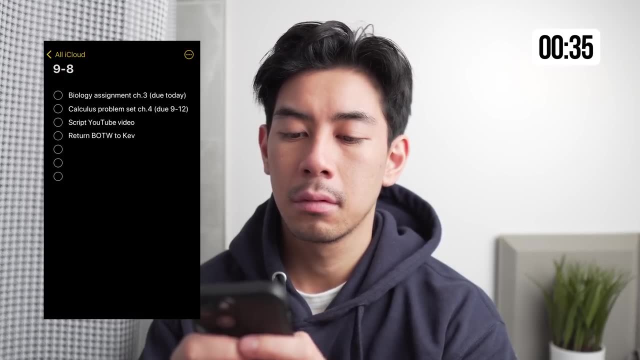 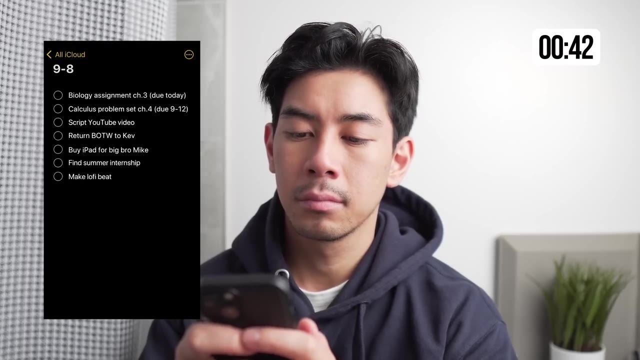 looks at all the tasks that need to be done: Biology assignment due today. calculus problem set due tomorrow. script a YouTube video. return Breath of the Wild to Kev or keep it and buy the DLC. buy his big bro Mike a new iPad for his birthday. find a summer internship and make. 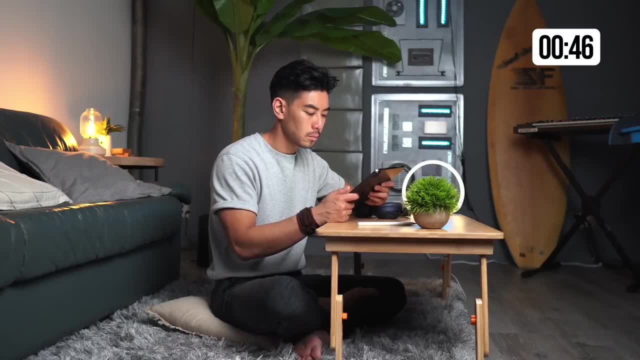 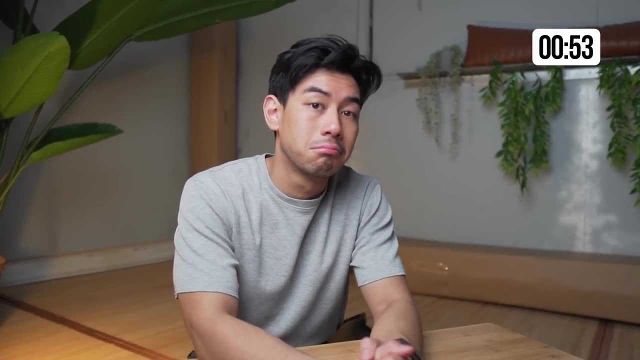 lo-fi beats for a study with me video. Now Maddie just needs to fit the most important tasks into the open slots. Luckily, Maddie has developed the skill of knowing exactly how much time it takes for him to do certain tasks, so this step is a breeze. He can finish the biology assignment and 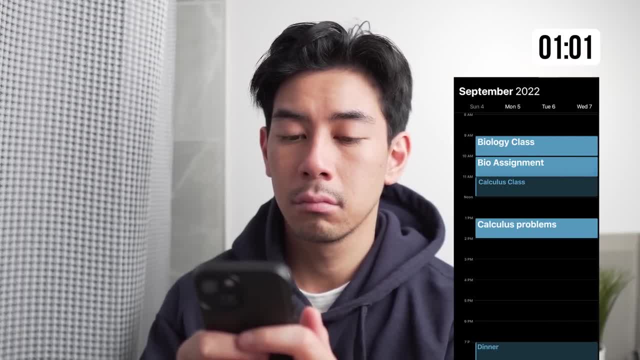 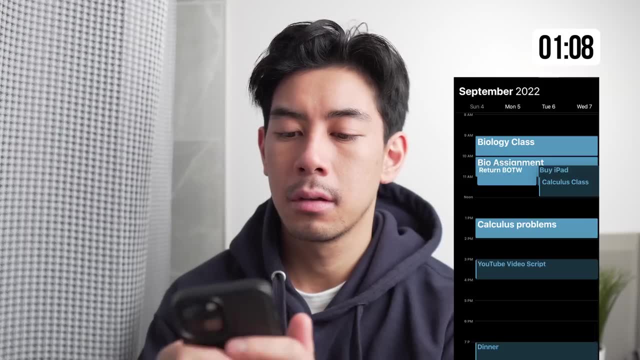 submit it in between class. He can also do some random chores in this hour, like returning the video game or slaying Ganon for the 50th time this week. It would likely take him about two hours each to do calculus and script the YouTube. 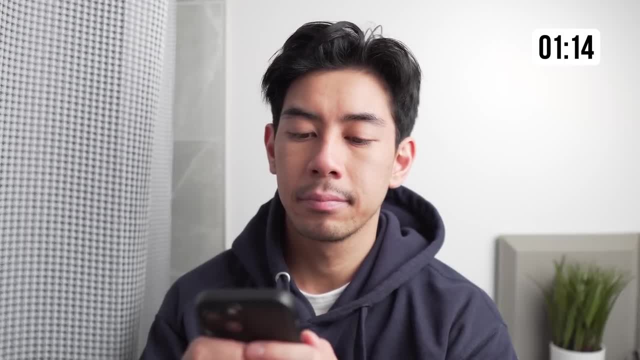 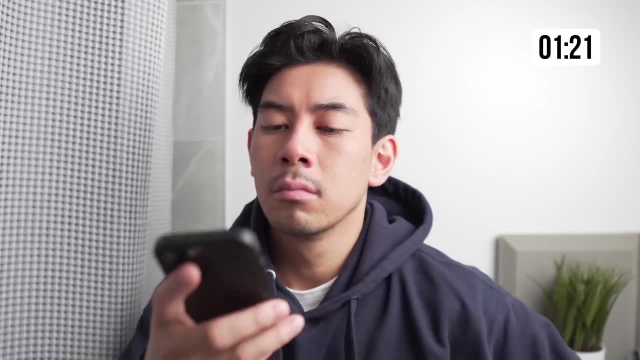 video, so he schedules them both after lunch. That takes him up to 5 pm and probably all the time he has for today. The other things on the list can get pushed to future dates because they aren't as urgent. And that's it. Maddie spent less than five minutes recording his task and